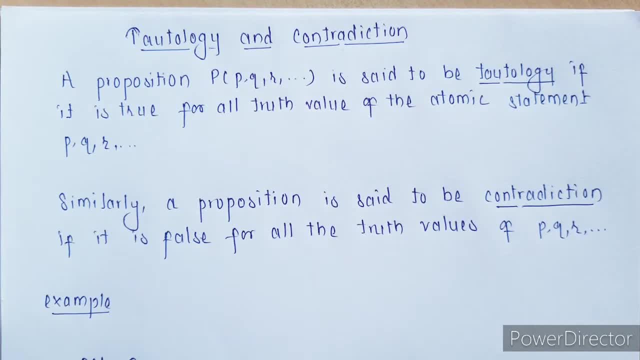 Last class we had discussed about logical equivalence. Now we will be discussing tautology and contradictions. First thing, tautology. So whenever, if given any proposition, suppose you are getting the final truth values, all the truth values, to be true, then that particular. 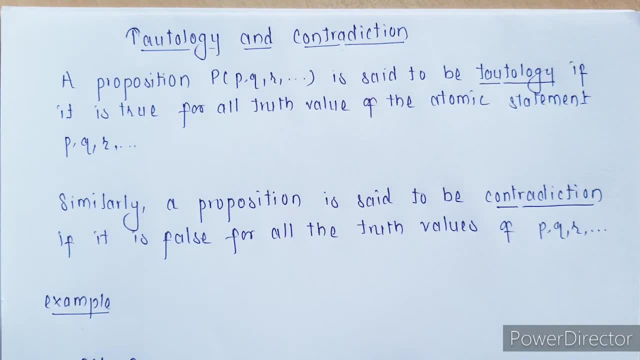 proposition is called as a tautology. And suppose: if you are getting all falses, all truth values to be falses, then it is called as a contradiction. If you are getting true as well as falses, then it is neither tautology nor contradiction. Okay, So let us look at 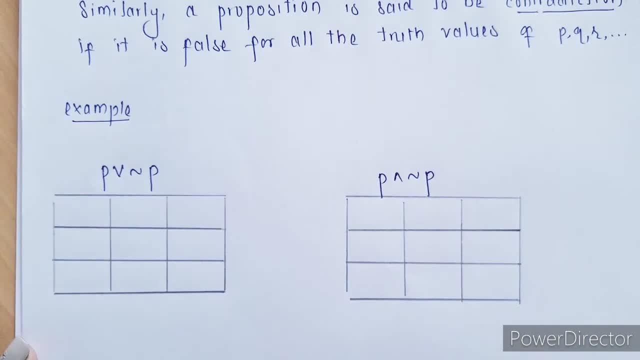 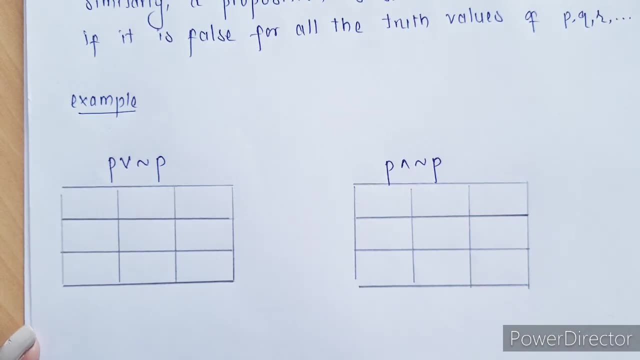 some examples Now. first one: what we have is P or negation of P. So since we have only one statement, that is P, there will be only two cases. Okay, So statement will be either true or false. Now we have P, we have to go for negation. 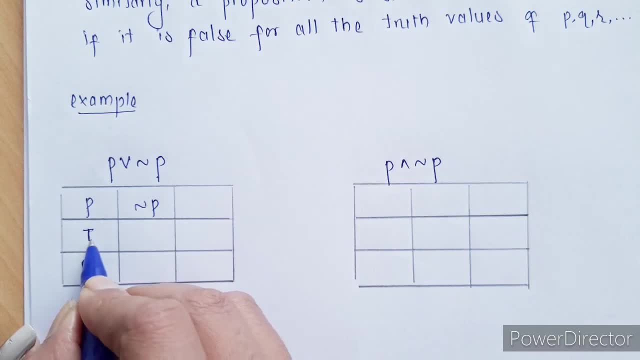 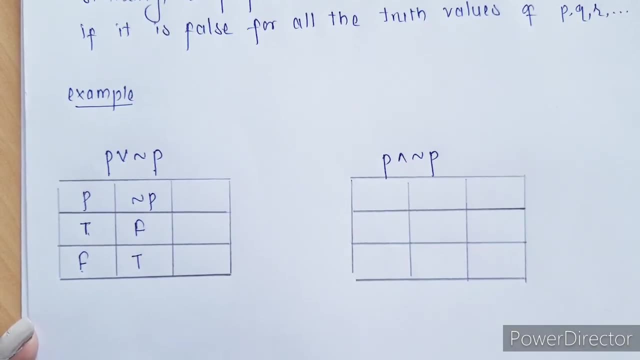 of P. So let us write negation of P. Since P is true, negation will be false. P is false, negation will be true. Next is we have to write P or negation of P. So, in case of or, 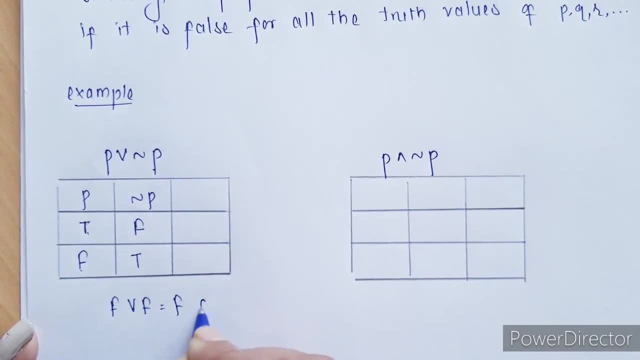 false or false is false. Otherwise, for all other cases, it is going to be true or false. So, true, true, that is right. P or negation of P: True or false, it is going to be true. 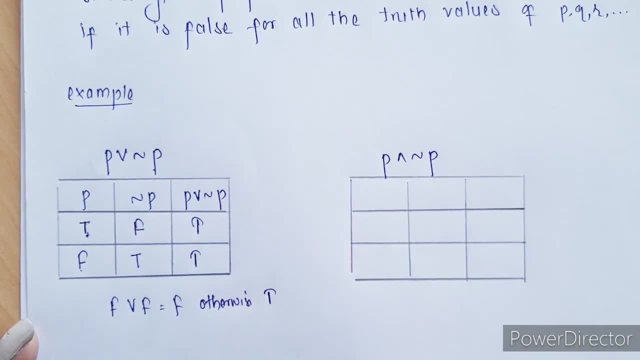 either are case And false or true also going to be true. Now, since this in this proposition, both are truths, all the values are true. this is called as a tautology. So this proposition, P or negation of P, is tautology. 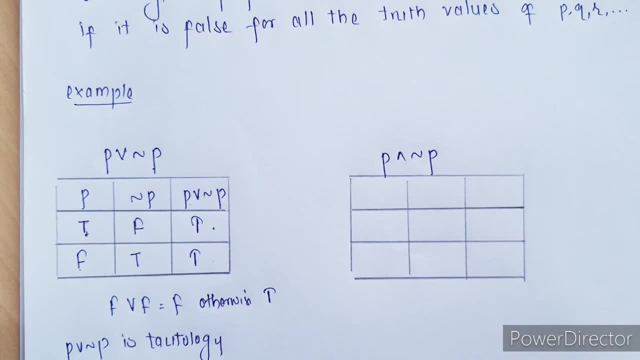 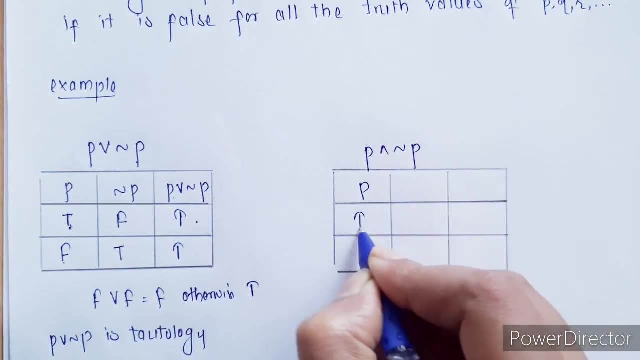 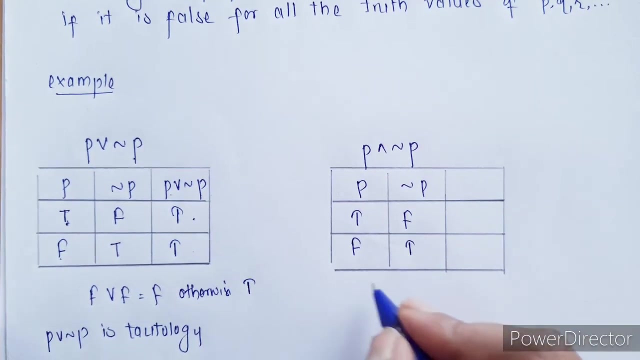 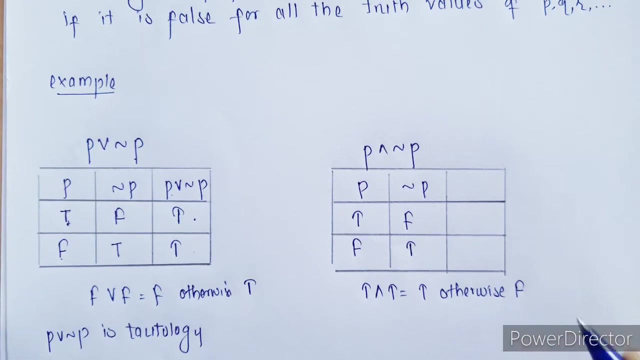 Okay, Next one: P and negation of P. So first let us write conditions for P is true and false. negation will be false and true Now in case of, and true and true is true. otherwise, for all other cases, it is going to be false. So, true and false. this is P and negation. 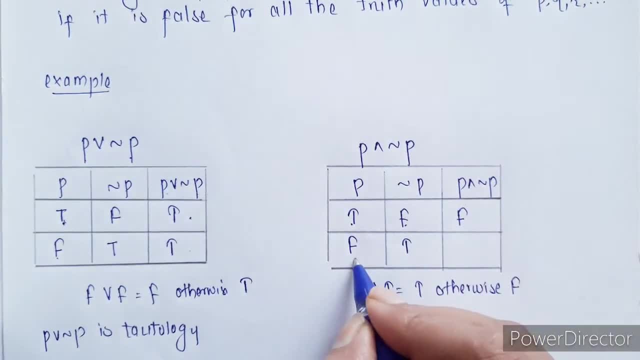 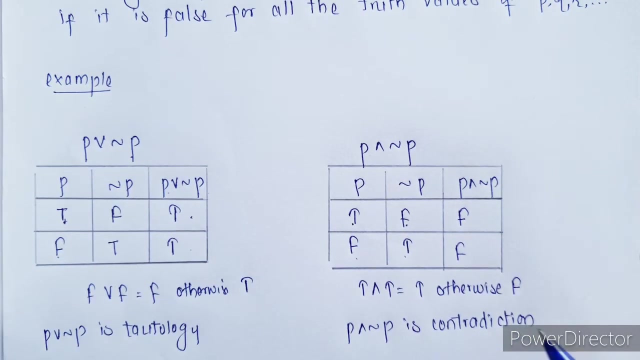 and negation of P. This will be false again. false and true will be false. Now, since both are falses, this P and negation of P is contradiction. ok, So if your final statement, that compound statement or proposition, if both all are, 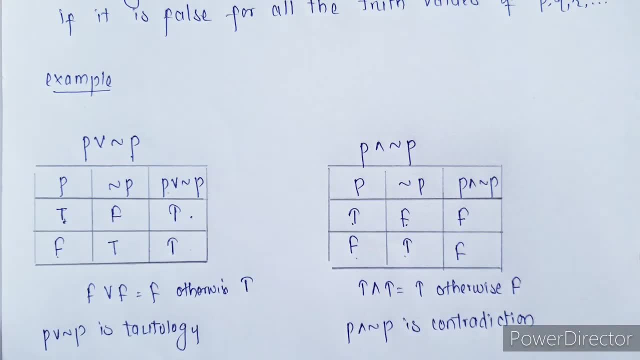 all the values are true, then it is called as a tautology. If all the values are false, it is called as contradiction. If you are getting mixed values, like you, are getting true as well as falses. so in such cases it is neither tautology nor contradiction. ok, 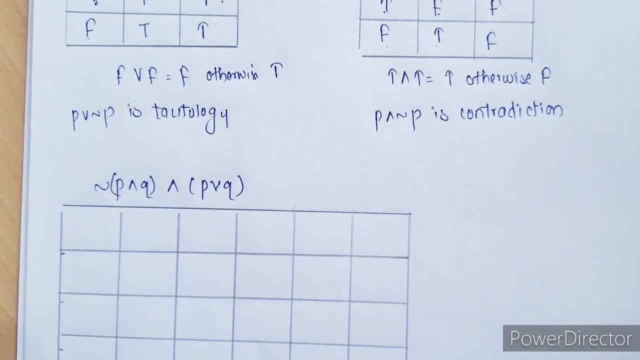 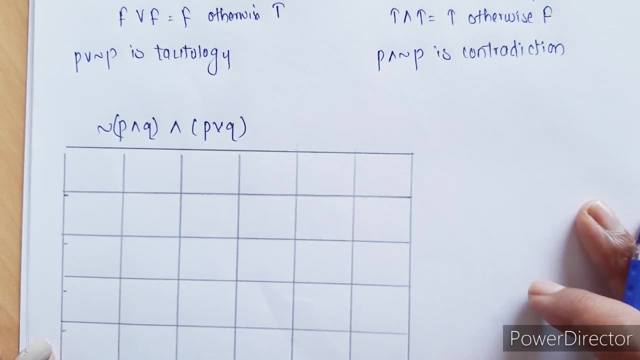 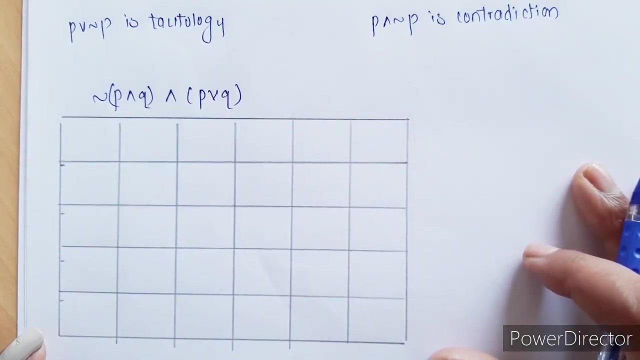 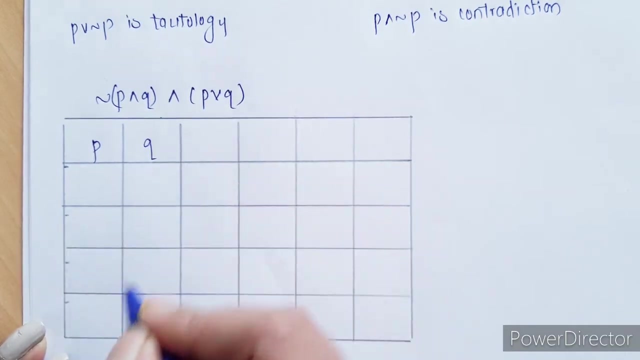 So let us move on to another example. So here we have to write truth table for negation of P and Q and P or Q. So we have to check whether this is tautology, contradiction or neither nor ok. So again, here we have two statements, so we have to write four cases, all possible. 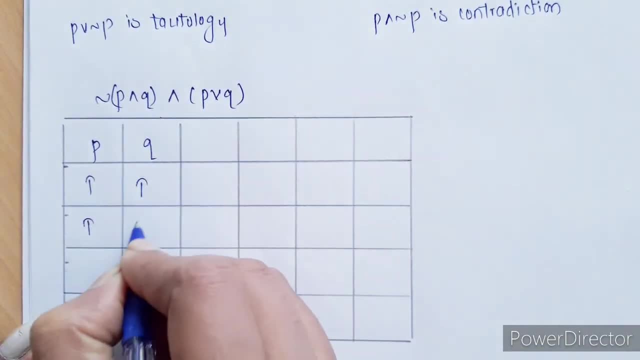 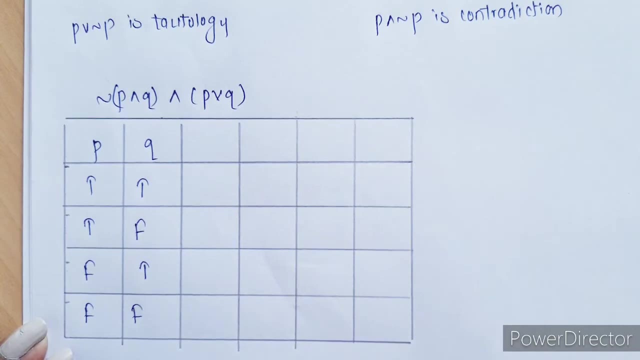 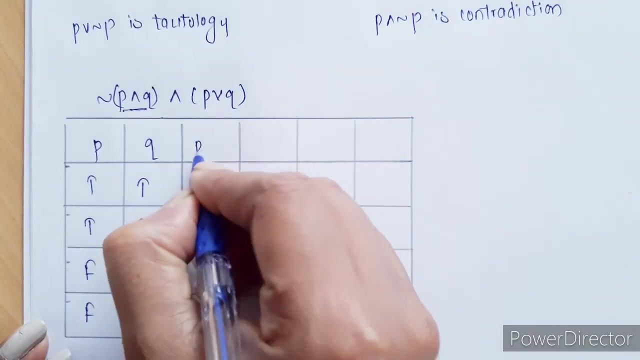 cases those are. both can be true, first true, second false, first false, second true, or both can be falses. Now, always start with bracket. so I am starting with this first bracket. In first bracket we have to find P and Q. Now in case of, and it is true and: 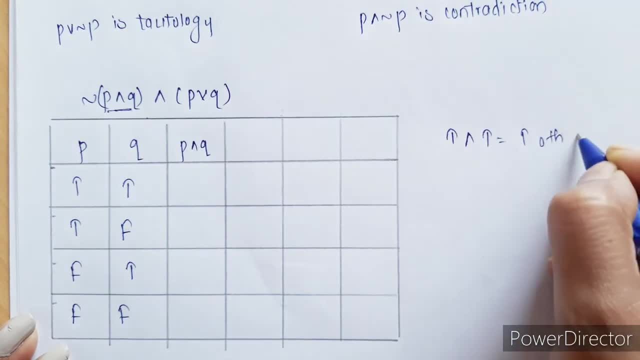 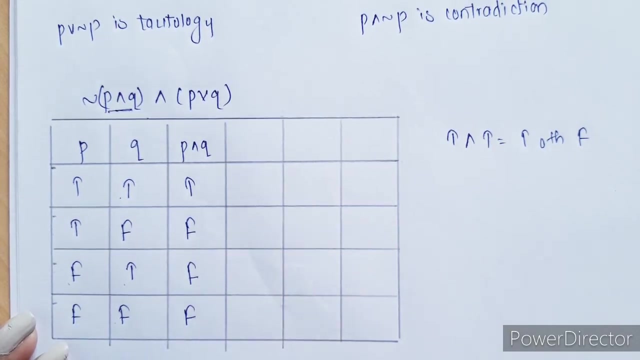 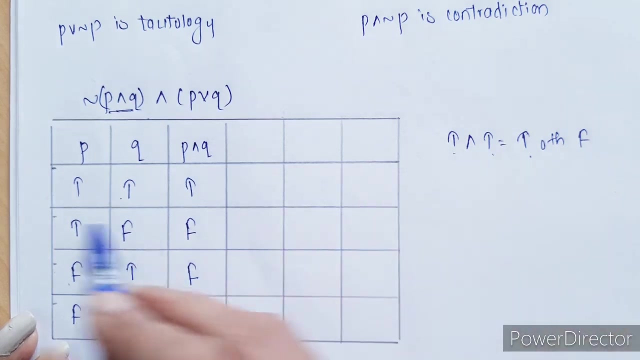 true is true, otherwise, for all other cases it is false. So, true and true. this will be true. true and false, false, false and true, false, false and false is again false. Only both are true, then only it is going to be true, otherwise, for all other cases it is false. 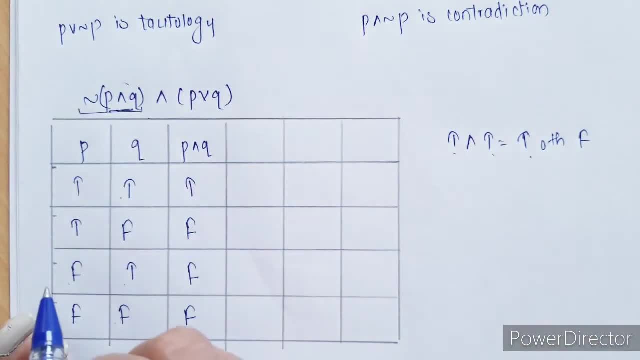 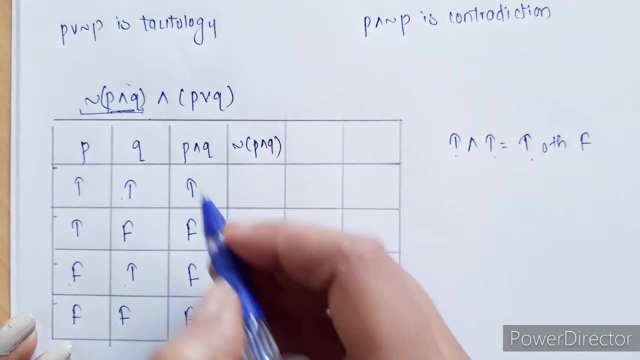 Now we got this bracket, let us move on to this complete compound statement that is negation of P and Q. So we have P and Q. where to find negation of that Opposite of that true? then this will be false, false, true, true and true. So we are done with this part, so we 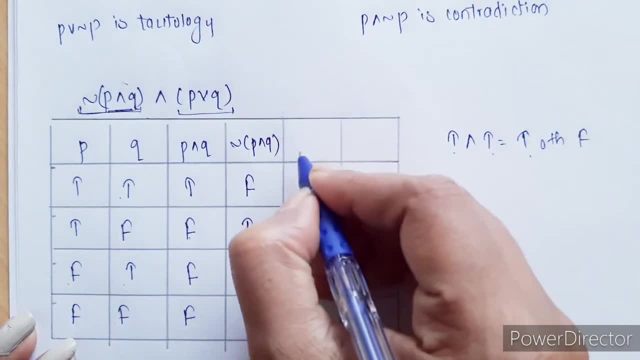 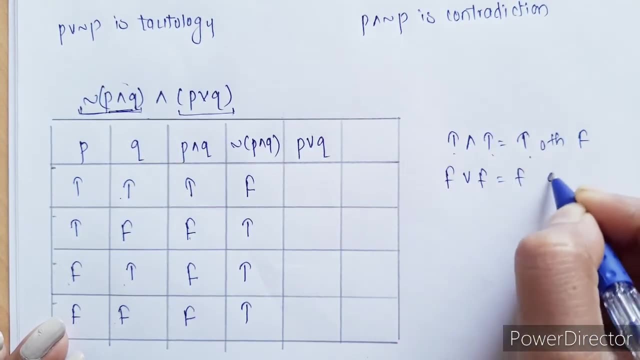 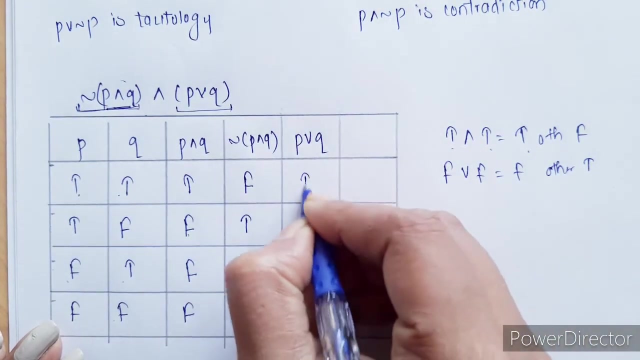 have to go for now. next bracket, that is P or Q. Now, in case of all false or false is false. otherwise, for all other condition it is going to be true. So true and true or true, true, true or false, true either. or condition: false or true again. 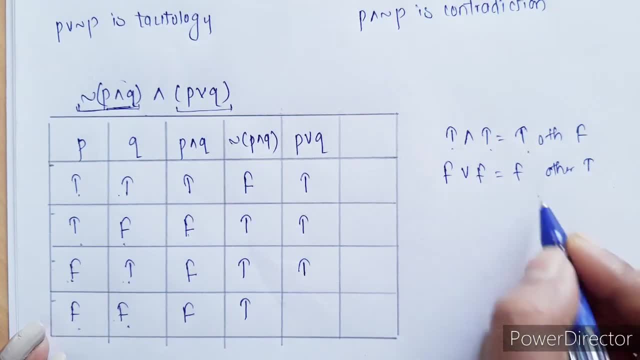 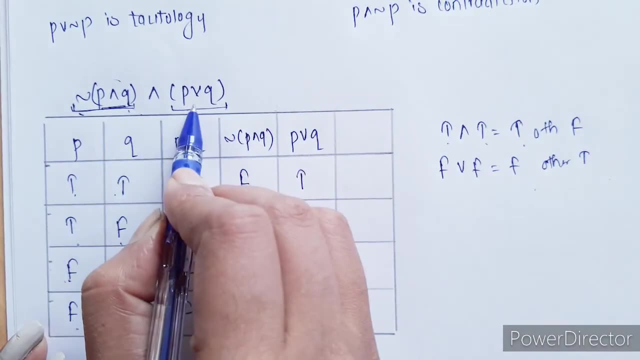 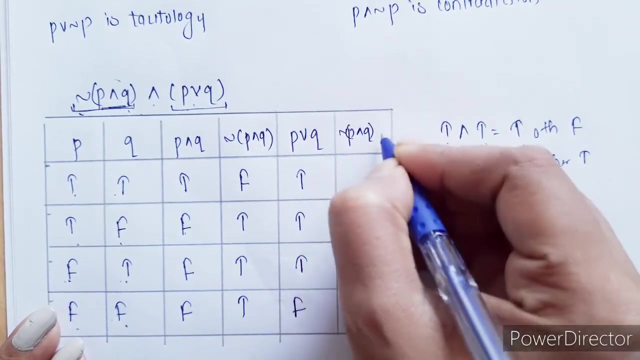 true either or condition false or false is going to be false. So we got this first part, we got even second part. now we have to connect both the compound statements using connective and we have to connect now negation of P and Q and P or Q. 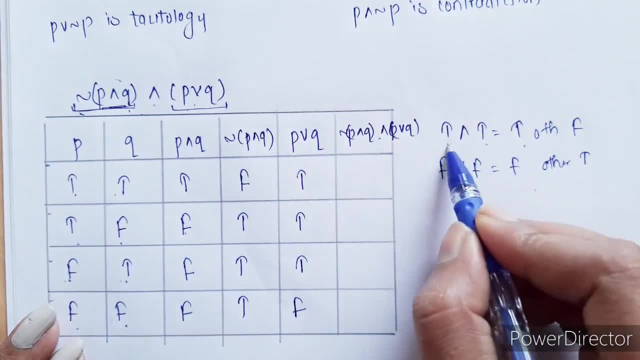 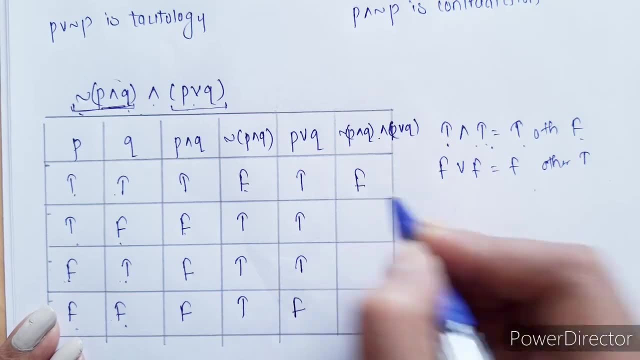 using connective, and so, in case of- and true and true is true. otherwise, for all other cases, it is false. So false and true, false, true and true. this is going to be true, true and true. this is true, true and false. this is false. 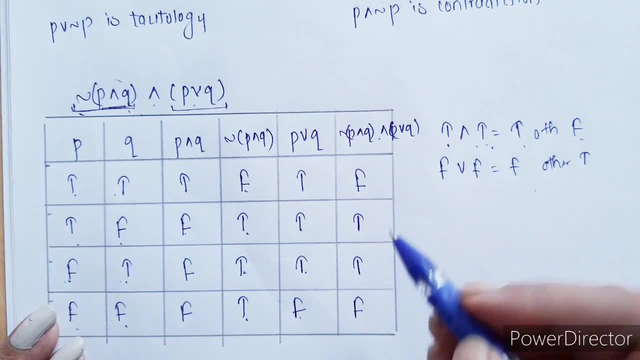 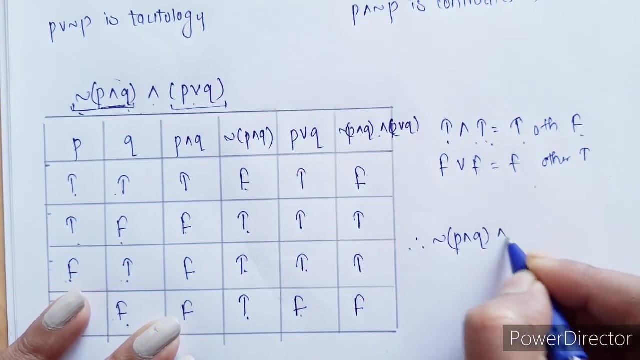 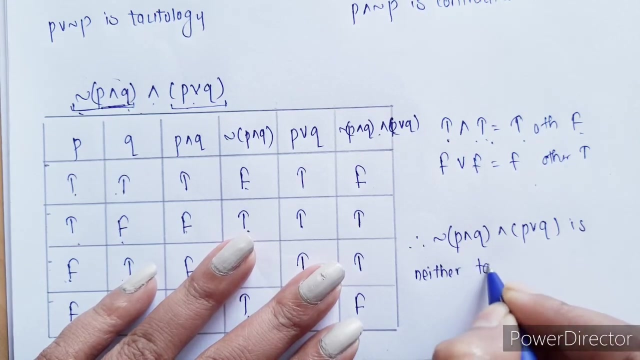 Now, in this case, we are getting falses as well as trues right, So this is neither tautology nor contradiction. So in this case, this is therefore negation of P and Q, and P or Q is neither tautology nor contradiction. So this is neither tautology nor contradiction.